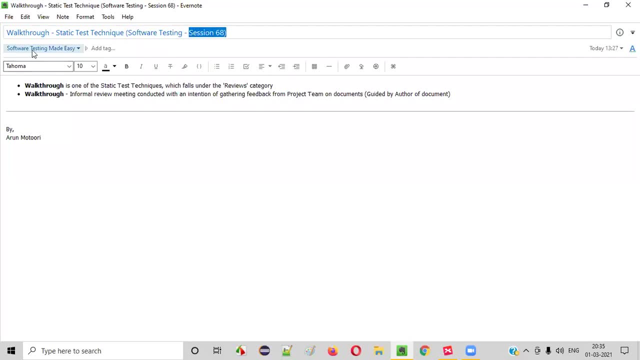 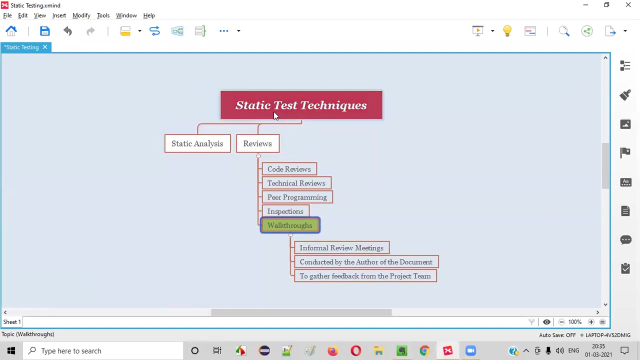 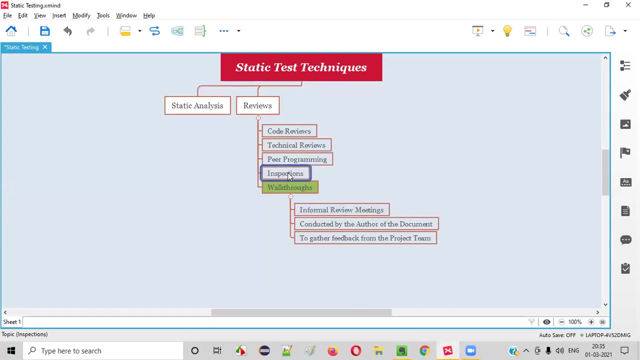 Hello everyone, Welcome to session 68 of Software Testing Made Easy course. In this session, I am going to explain one of the static test techniques, that is, walkthroughs. So let's get started. What exactly are these walkthroughs? Walkthroughs are one of the static test techniques. As you can see here, static test techniques can be categorized at a high level into static analysis and reviews. Under reviews, we have subtypes like code reviews, technical reviews, peer programming inspections and walkthroughs. 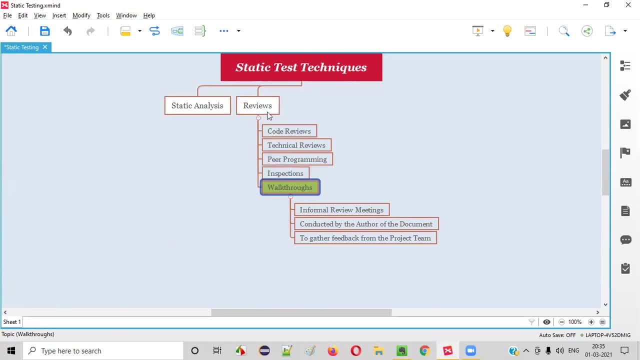 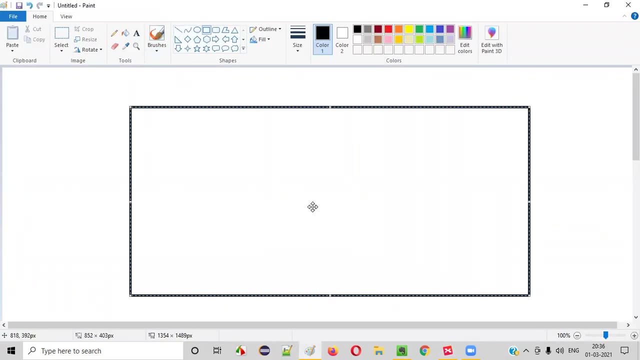 But what exactly are these walkthroughs? Walkthroughs are a type of reviews, guys, which are nothing but informal review meetings which are conducted by the author of the document to gather feedback from the project team. Let me give an example. Let's say there is a project, guys. Okay, In this project, one person say BA. let's say there is a person BA- business analyst. he created one document- BRS document. Now, what this person does is he will conduct some informal meeting. Okay, this BA person will conduct some informal meeting with all the other team members in the project. The team members may include testers. 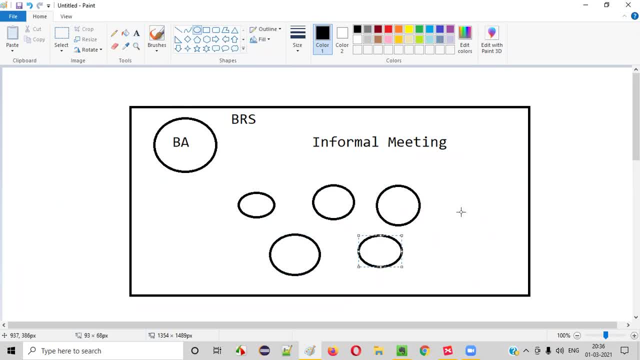 developers, architect, project managers- okay, development managers, testing managers, whatever it is. okay. all the team members will gather in this informal meeting and this BA person will present this BRS document, okay, Okay, we'll showcase this BRS document to all the team members. What will happen when all the team members will review this BRS document? They'll start reviewing, okay. they'll point out the mistakes or ambiguities if they are not understanding anything, or they will raise the questions. they'll ask the doubts about this. 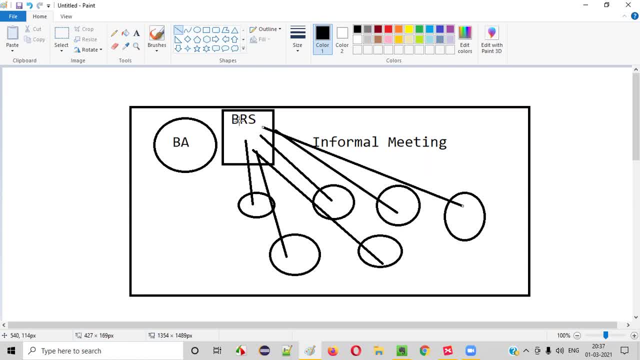 BRS document. What here? this BRS document is created by BA guys, So BA is the author here, The author of this document, In this case, for this BRS document. who is author? BA Tomorrow, for test cases document, who will be the author, The test lead or someone like that? So the author? 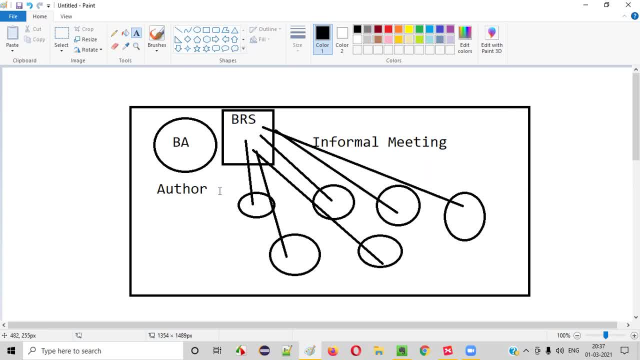 of the document will conduct some informal meeting where all the other project team members will attend that meeting and will start reviewing the document. While BA is presenting this document to all the team members, all the other team members will point out the mistakes, ambiguities and they.